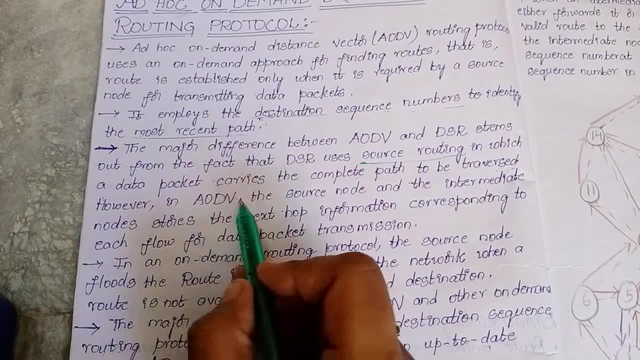 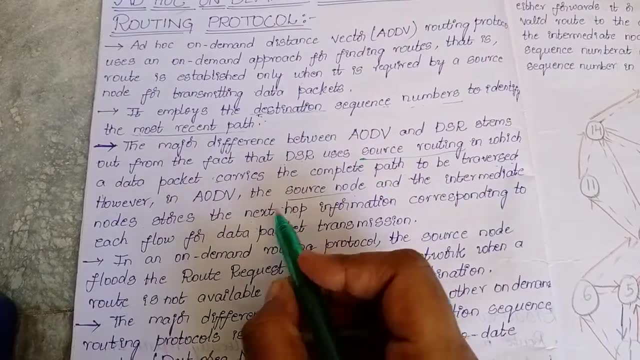 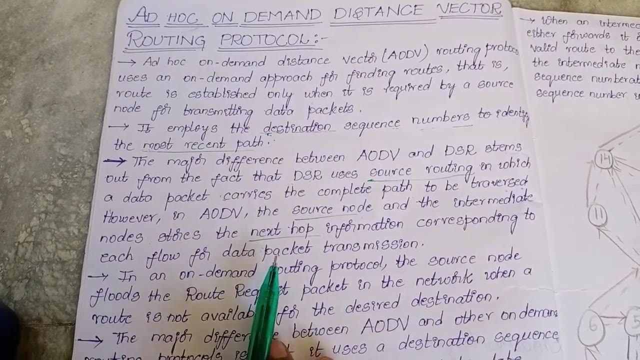 to be traversed means the route will be in that data packet. However, in AUDV, the source node- source node and the intermediate node- stores the next hop information. Next hop means whether it may be single hop or double hop. it stores the neighboring nodes, information corresponding to each flow for 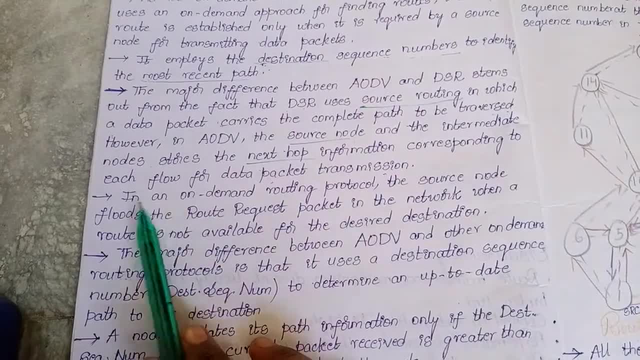 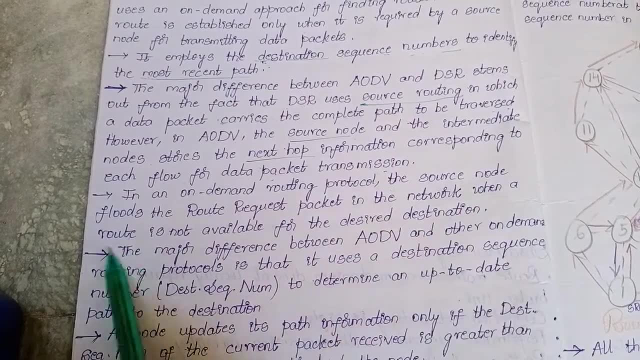 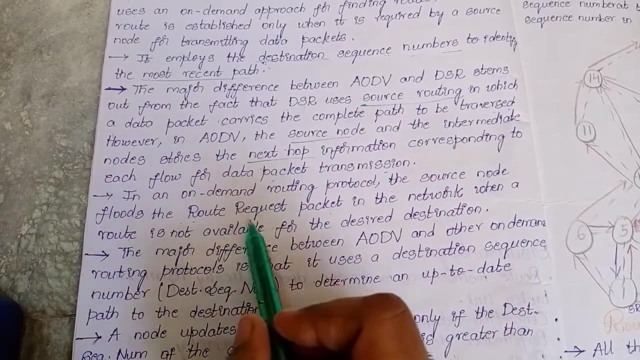 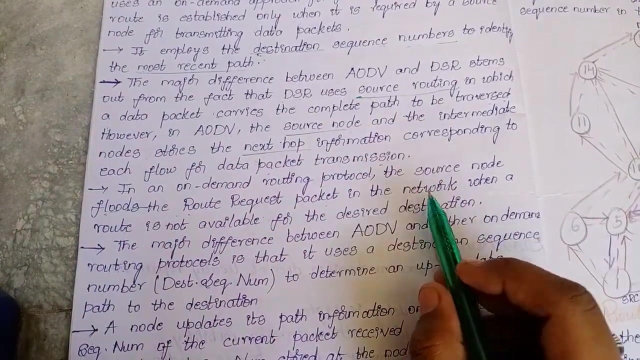 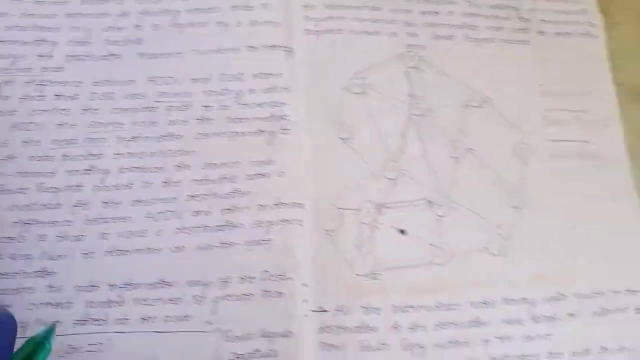 data packet transmission In an on-demand routing protocol. the source node. in an on-demand routing protocol, the source node floods the route request packet. Route request packet means it will request all the neighboring nodes and this flooding means it the source node will just send the route request packet to all the nodes in its network. I'll explain you how, for example: 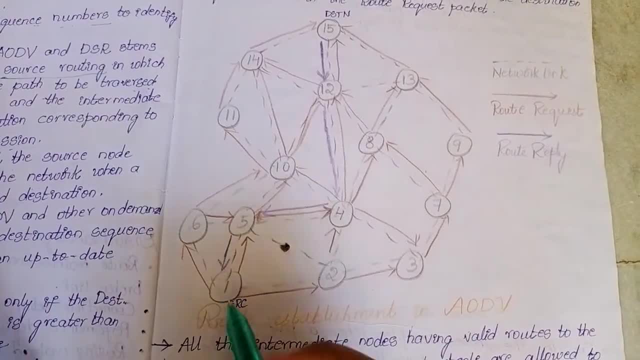 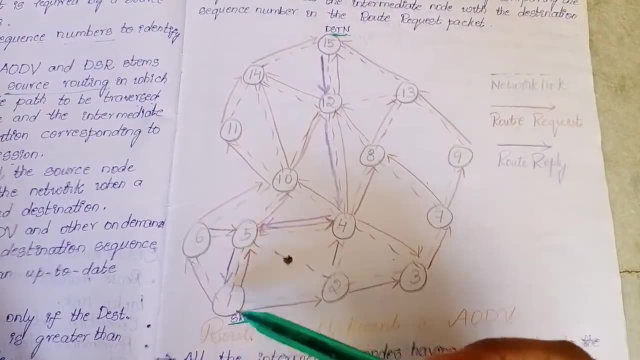 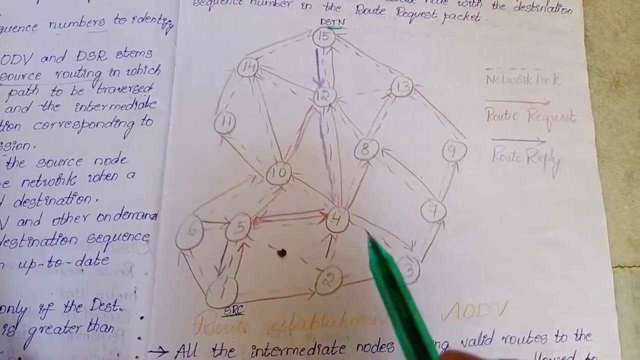 let us consider here: our source is node 1 and our destination is node 15. we don't know that, I mean we not know the route from source node to the destination node, right. so in order to find the route, the source node will send the route request packet to all the 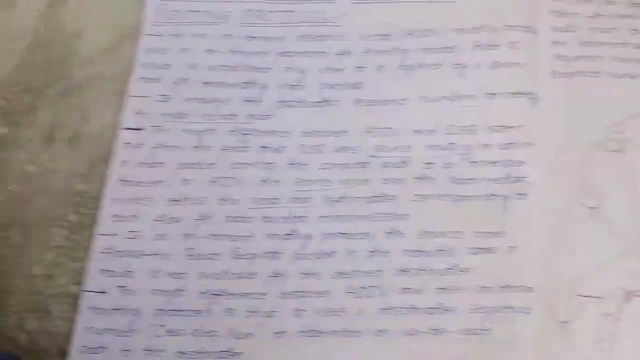 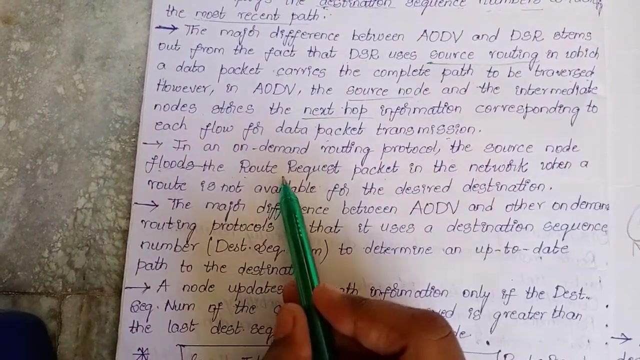 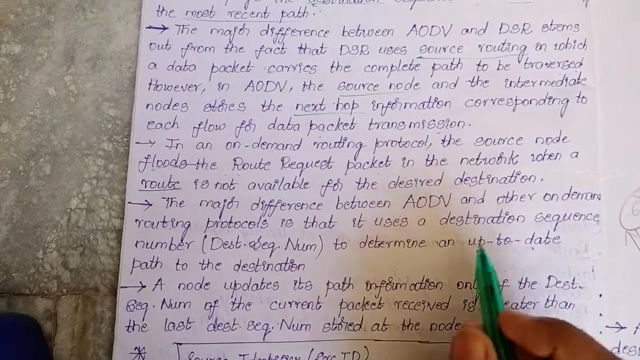 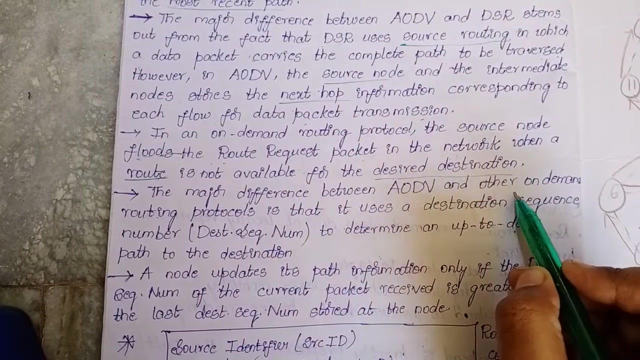 nodes in this network. that is flooding back to the concept. it floods the. the source node floods the route request packet in the network. when a route is not available, then there is no route, then only it floods for the desired destination. the major difference between a o DV and other on-demand routing: 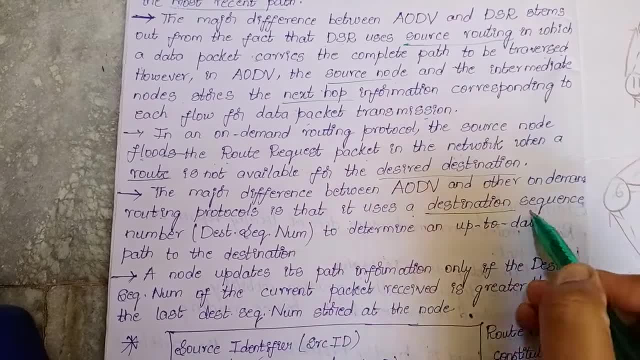 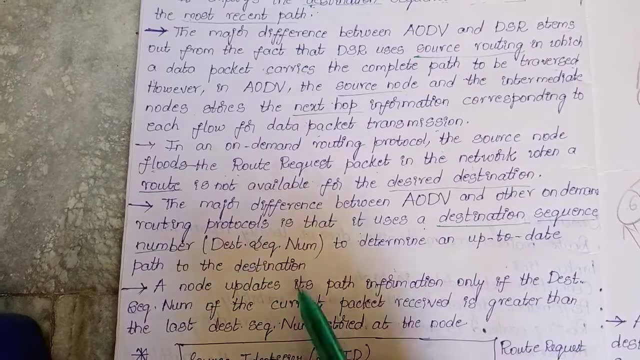 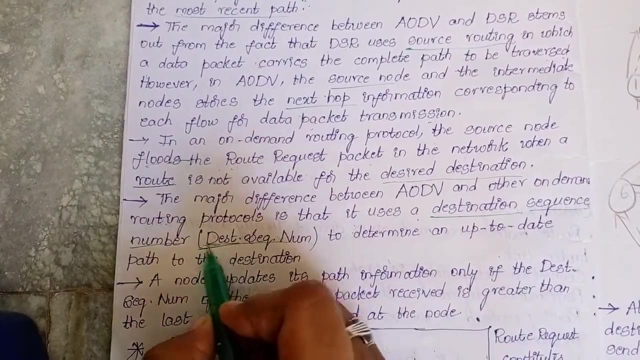 protocols is that it uses a destination sequence number. no protocol in this on-demand routing protocols we use this destination sequence number. I mean some protocols such as the DSR will use sequence number, but it is not destination number. it is not destination number. it is not destination number. it is not. 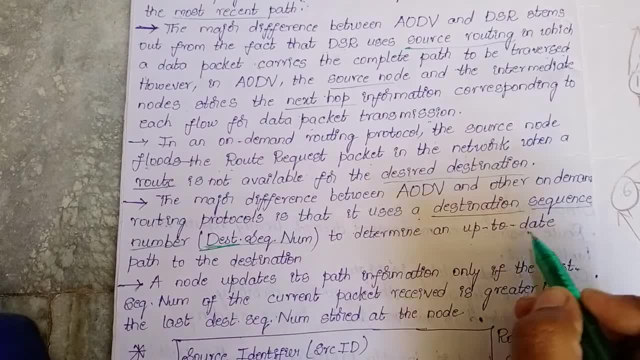 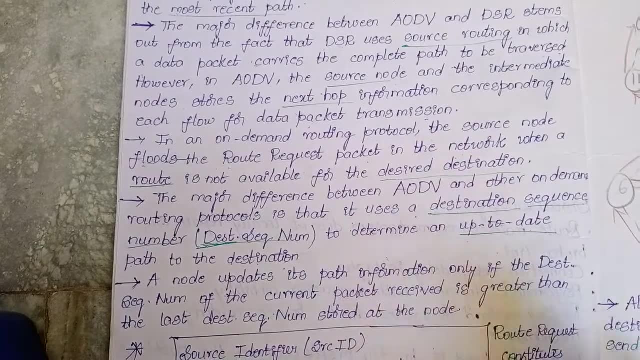 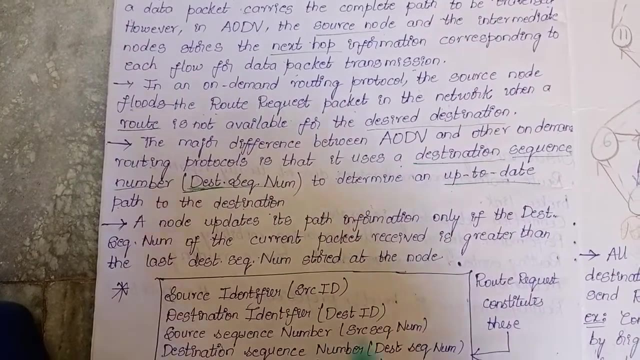 sequence number. this is a point to remember to determine an up-to-date path from the path to the destination. up-to-date path. in the up-to-date path indicates such as it must be valid, there must not be any path breaks or broken links in between them, in between the source and the. 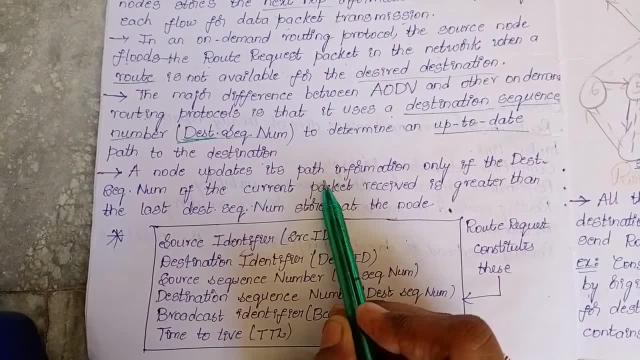 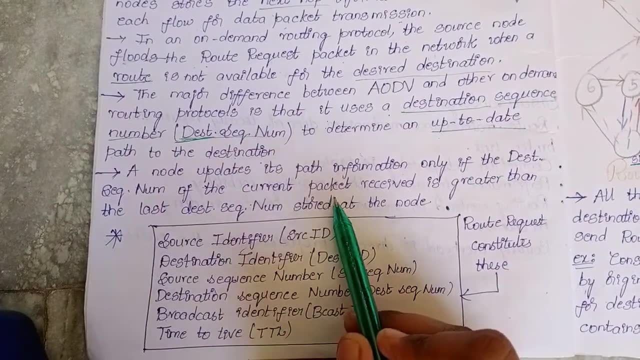 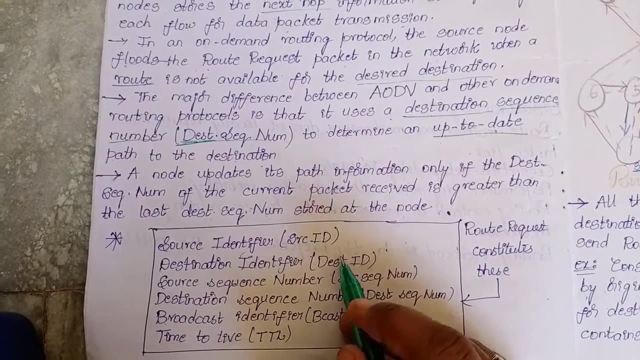 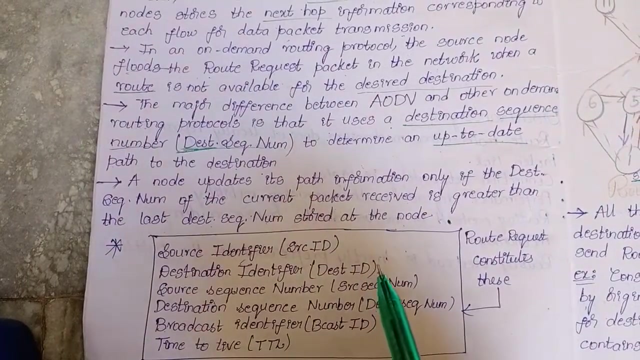 destination a node updates its path information. a node updates its path information only if the destination sequence number of the current packet received is greater than the last destination number stored at the node. as i have already told you the destination, i mean the sequence number. normally the sequence number must be highest, must be the greatest one when a node receives a packet. 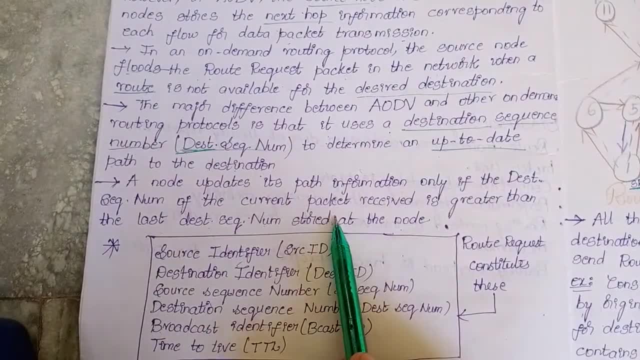 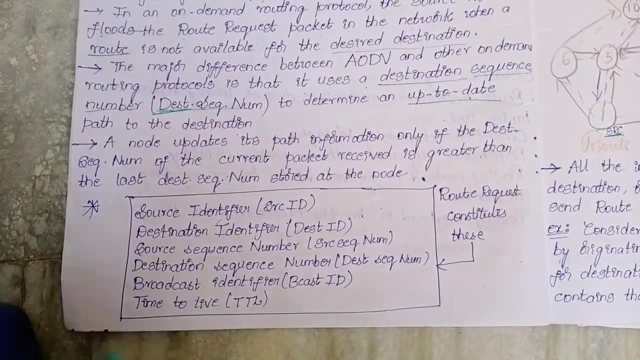 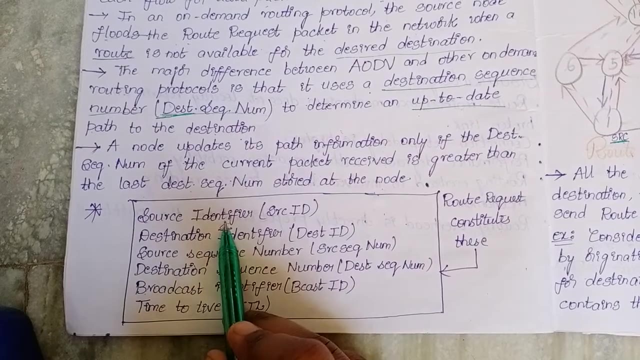 here the destination sequence number of the current packet must be greater than the last. i mean past received packet. here is the information what root request constitutes. root request generally constitutes of the source identifier. i mean address or something which is related to source. in order to identify a source, we will have 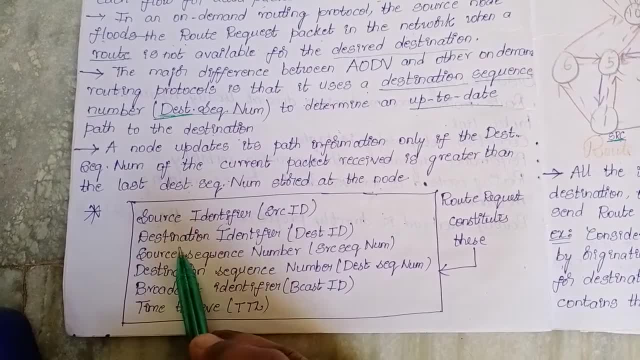 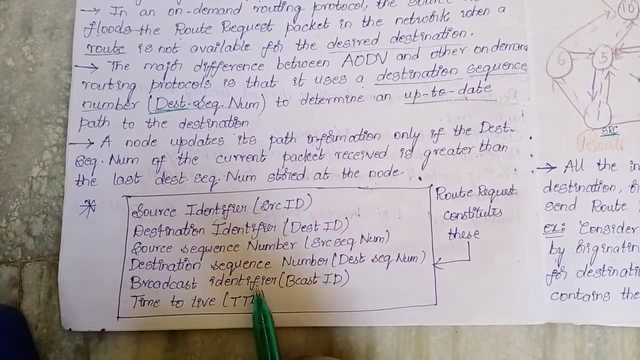 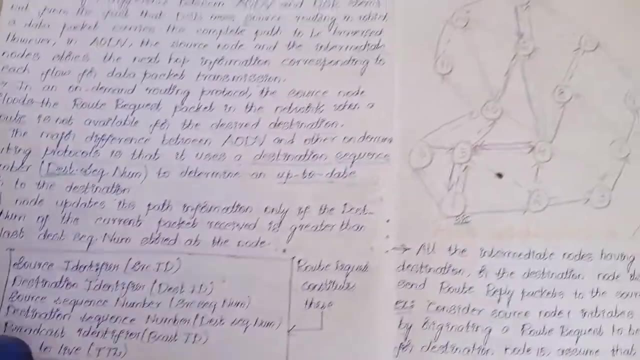 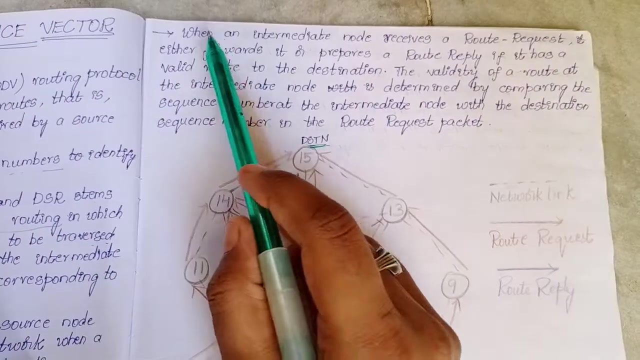 address. that is here. source identifier, destination identifier. address of the destination. source sequence number, destination sequence number, broadcast identifier- time tooling. i'll explain each and every point later. please be with me. when an intermediate node receives a root request: when an intermediate node means the node which is: 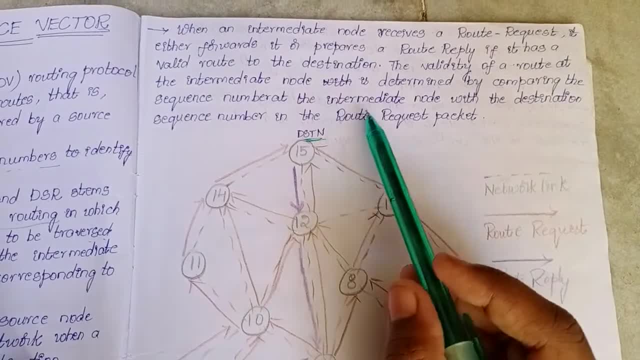 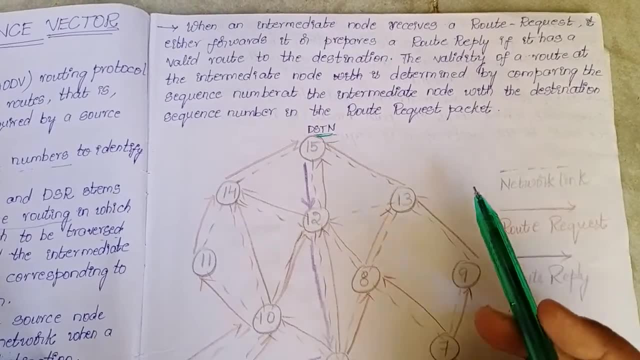 in between the destination and this source is known as intermediate node. here, 12, 10, 8, the- these nodes are intermediate nodes. when an intermediate node receives a root request, it either forwards it or prepares it to receive a root request. when an intermediate node receives a root request, it either 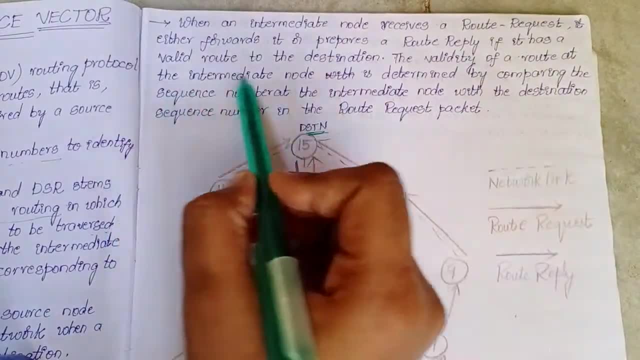 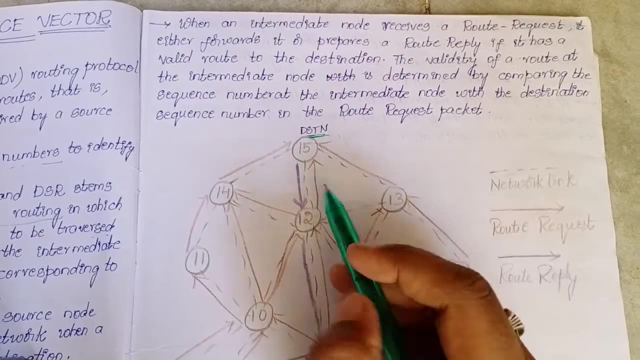 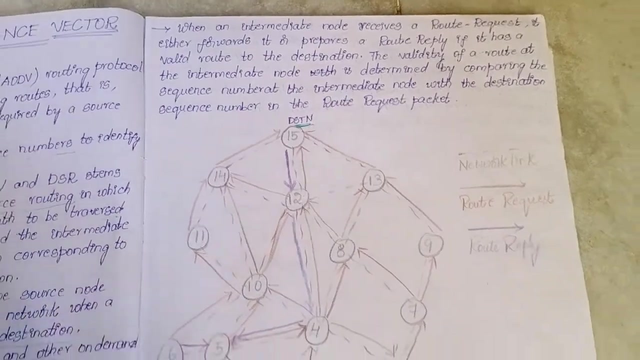 is the root reply packet if it has a valid route to the destination. if it, i mean if the intermediate node has a valid route to the destination, then the intermediate node itself sends the root reply packet to the source node. did you get my point? i'll explain it with an example. here we have this: 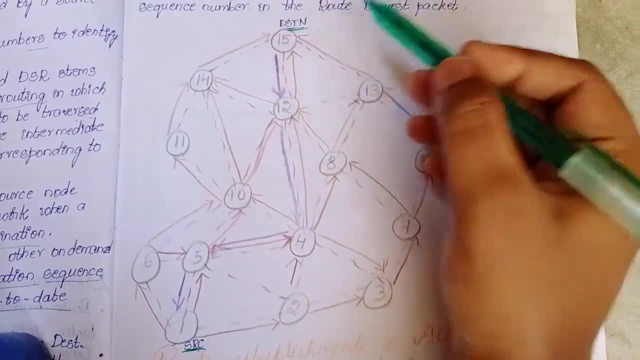 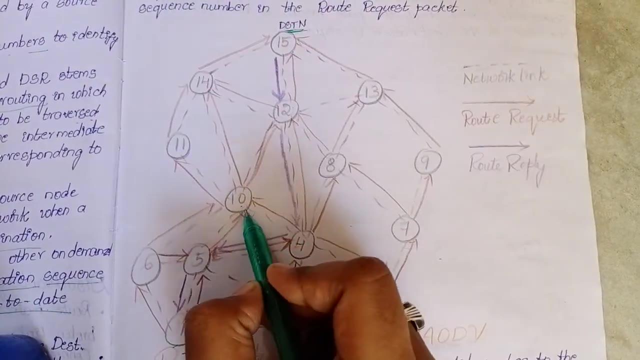 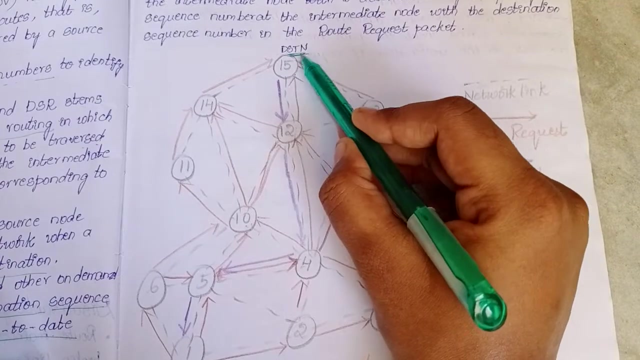 source node 1. right destination node 15. if this intermediate node 10 has a valid route to destination, then this intermediate node 10 itself sends the root reply packet to the source node. actually the root reply packet must be sent from destination. but in aodv if any intermediate nodes 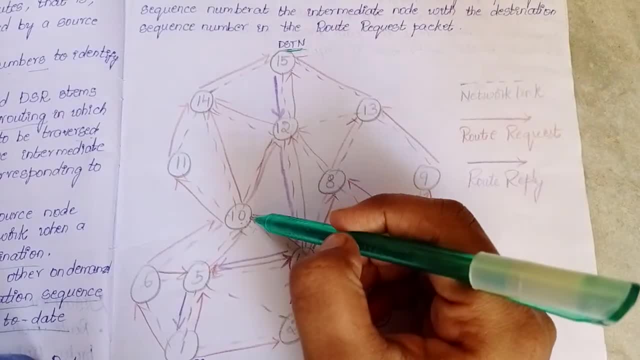 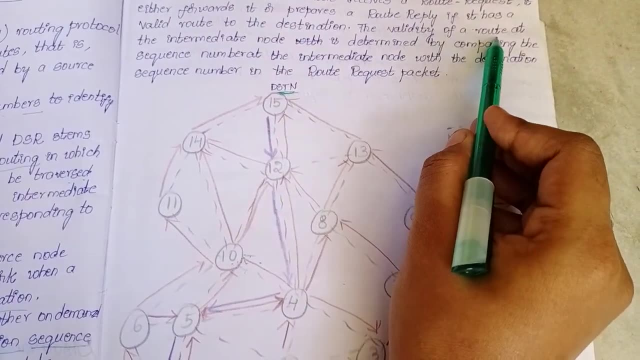 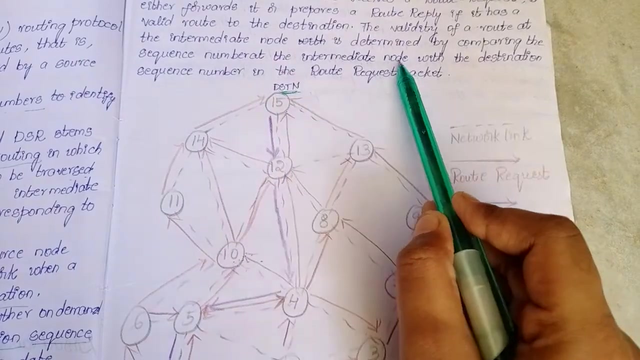 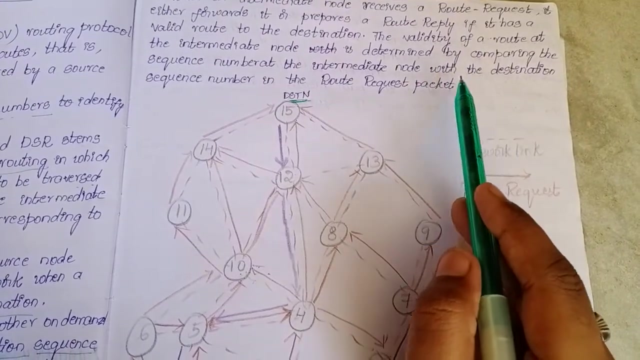 has a valid route to the destination, then it can also send this root reply to the source. see, the validity of a route at the intermediate node is determined by comparing the sequence number. you have sequence number at the intermediate node with the destination sequence number in the root request packet. as i have already told you, up to date information validity will be done. 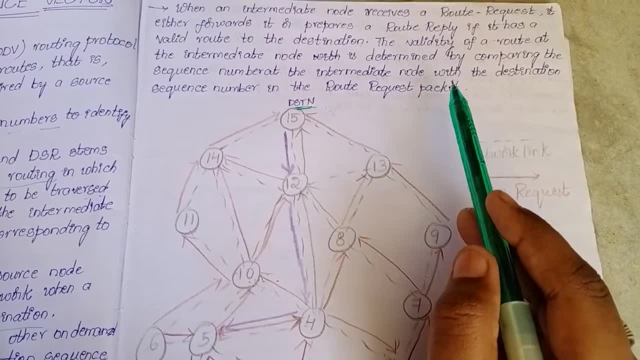 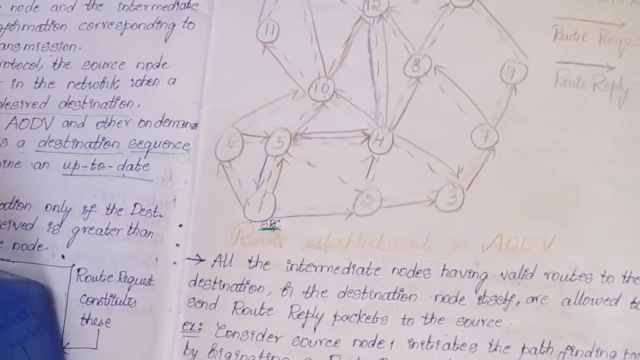 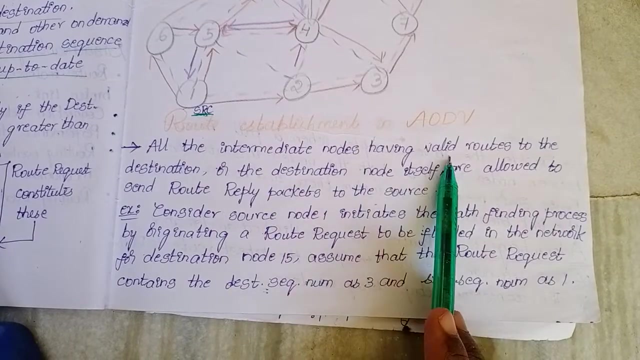 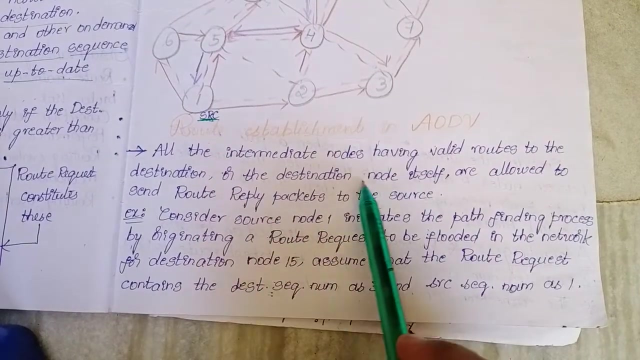 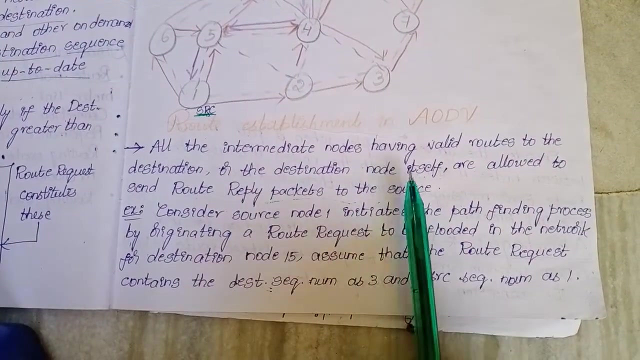 by using sequence number, the highest, the sequence number, the fresh one, it is generated, the fresh one. all the intermediate nodes having valid routes to the destination, all the intermediate nodes having valid routes to the destination or the destination node itself, are allowed to send the root reflect packets to the source. as i have already told you, this happens. 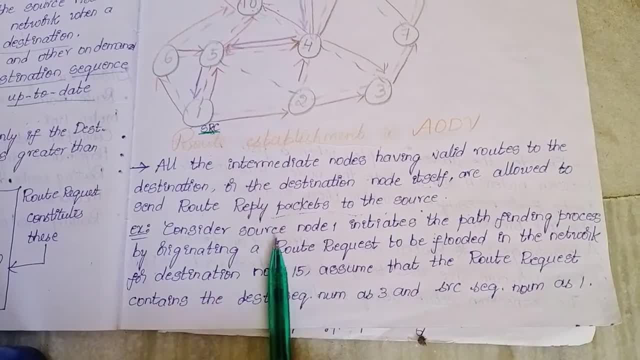 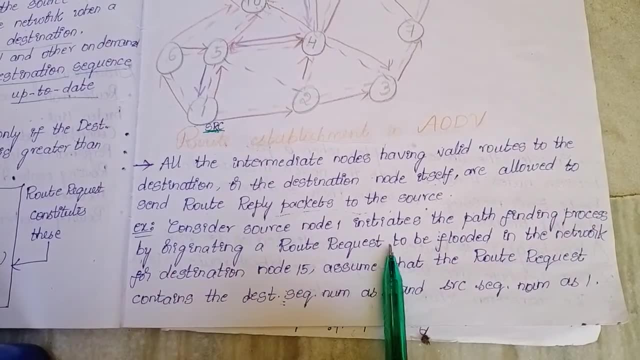 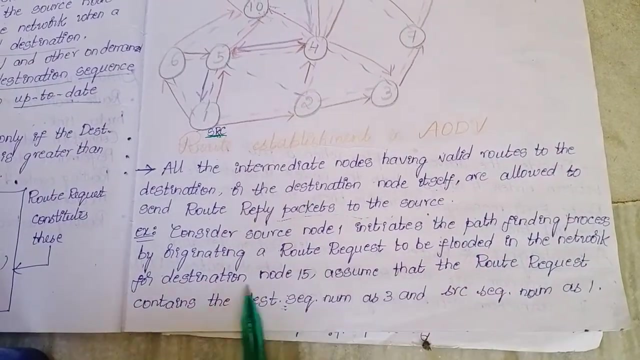 only in aodb, not in any other protocol. consider source: node 1 initiates the pathfinding process. pathfinding process means it will generate the root request packet means, by originating a root request, to be flooded in the network for destination node 15. assume that the root. 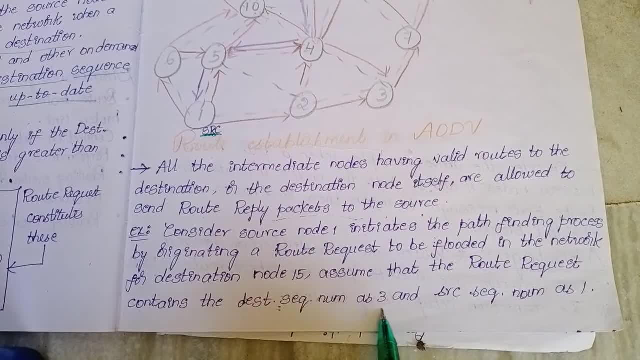 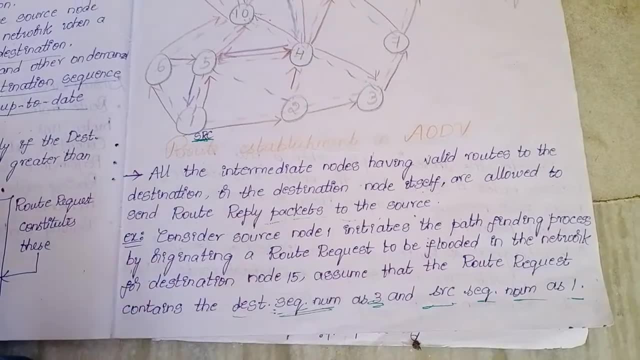 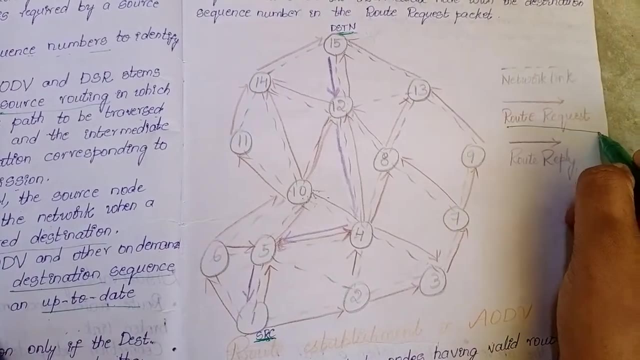 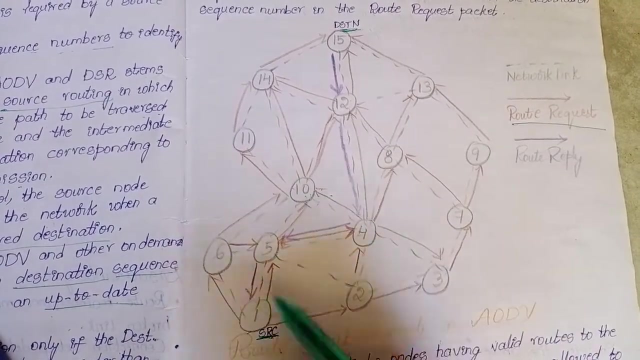 request contains the destination sequence number, as 3 means. here the destination sequence number is 3 and the source sequence number is 1: see here the source node has generated root request packet. see. it has generated root request packet and it is flooded throughout the network. see. it has sent to all its neighboring nodes. 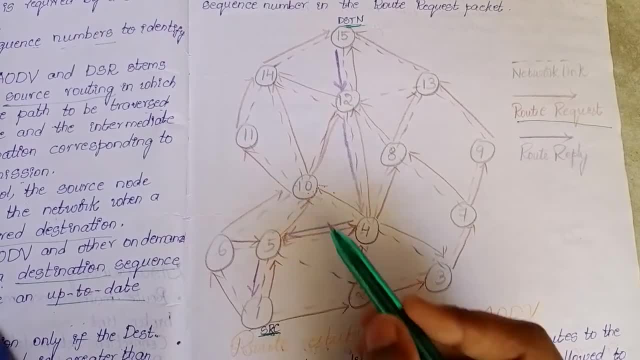 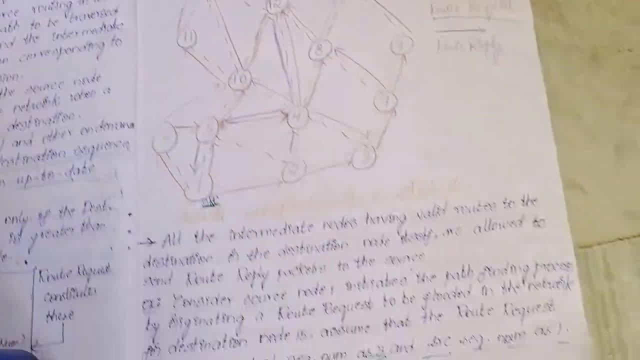 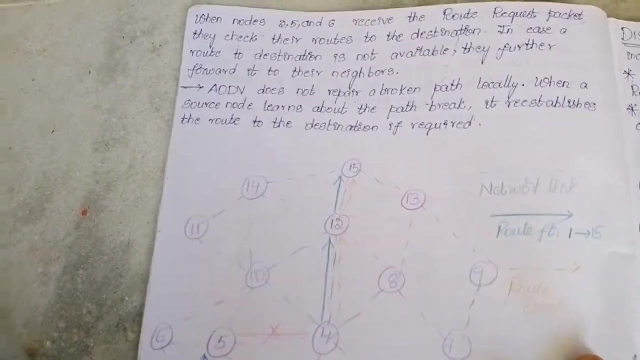 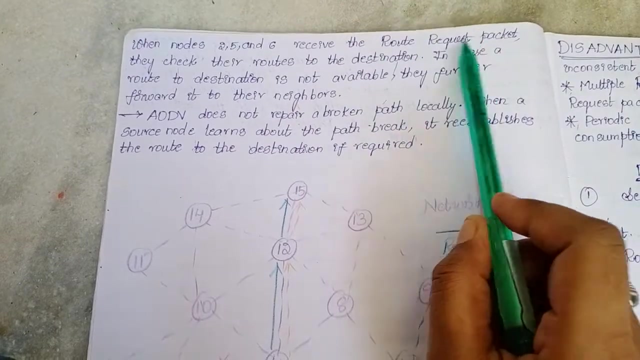 6, 5, 2 they have sent to their neighboring nodes. this is made by flooding and the destination sequence number is 3 and the source sequence number is 1. then nodes 2, 5 and 6 receives the root request packet. they checks their roots to the destination. 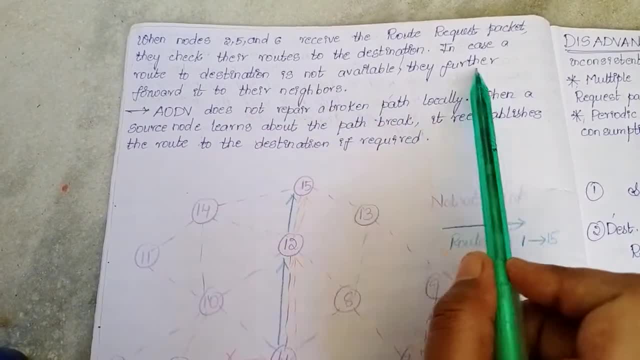 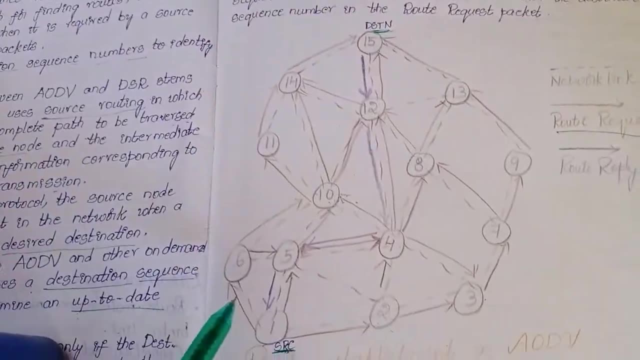 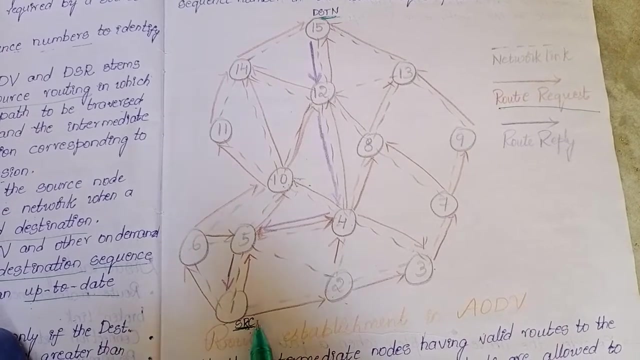 in case a root to the destination is not available, they further forward it to the neighbors. this means- i will again explain with this example: see here. in order to initiate the pathfinding process, the source node has to originate the root request packet. this source node will send the root request packet to its neighboring node. 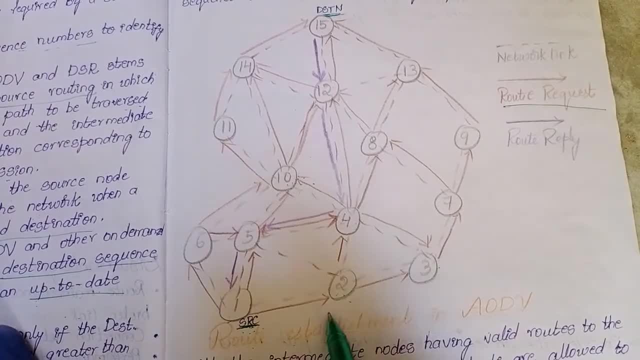 5. its sources node will forward the root request packet to its neighbor. this is called for. IE noted that similarly at the source node. the source node is Wennuts by related die fallen rooted to the destination directly. 5, quickly we will go to system nodes 2 by 6. if IE had simple route, uh, IE nodes 2 by 6. 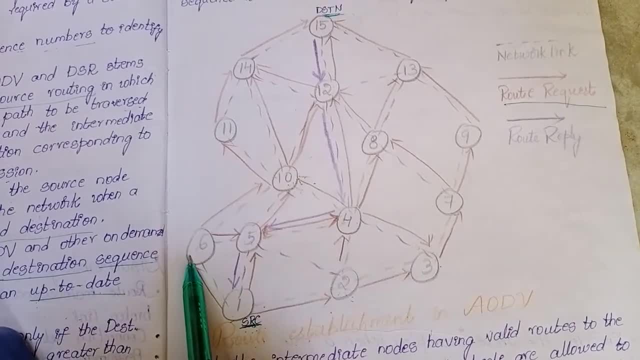 it used to have type of a type IE nodes: 2 by 6 by 6. no, it was made a Node 2 by 5 and IE is expected to haveulty right now if the rack is will send the root recommend packet. явility nodes. that is flooding. the flooding happens here. questão: fruit request packet. 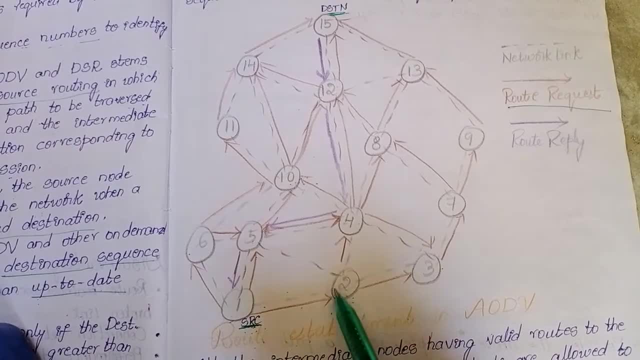 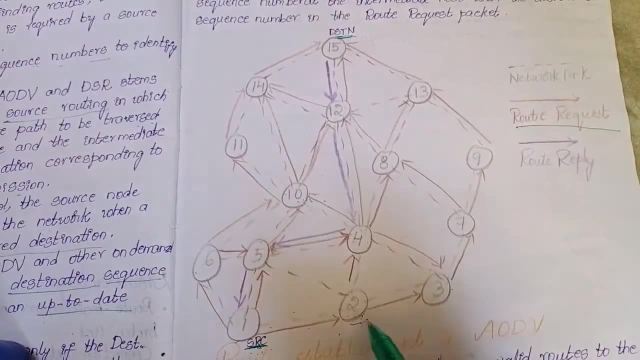 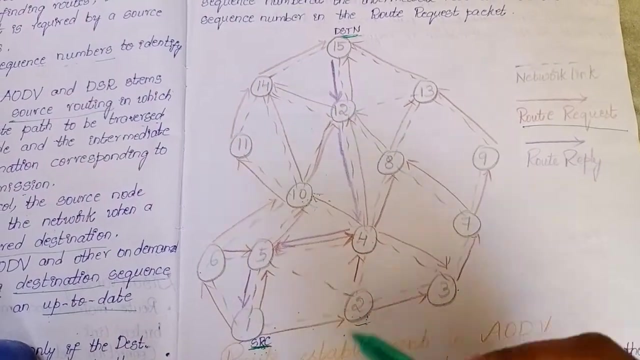 8 will be sent to nodes 2, 5, 6. in this example, when nodes 2, 5, 6 don't have a valid route to the destination directly, then these intermediate node will forward the root request packet to its neighbors. if it has a valid route to the destination, it will send root replay a. 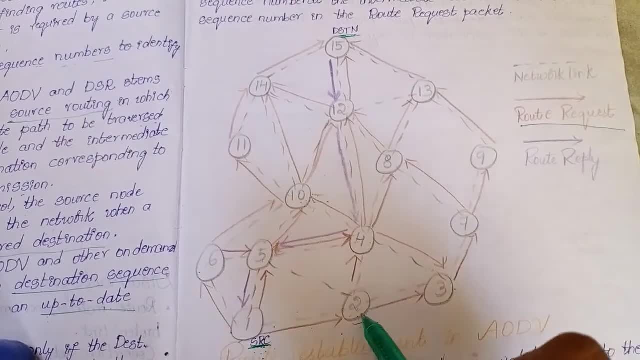 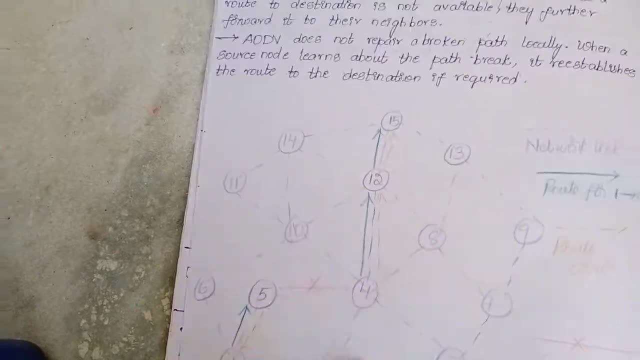 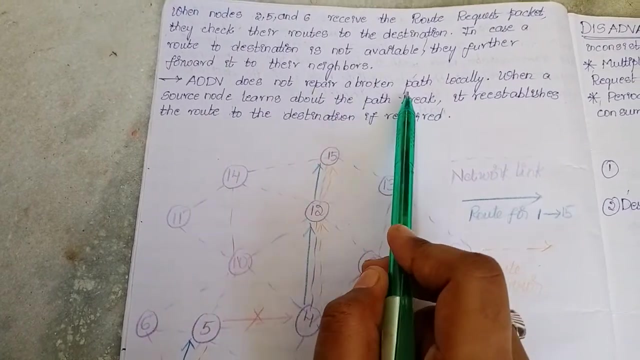 shortcut to the source node, otherwiseअ it will not receive thebabblej same白 severa this source node, otherwise it will forward the route request packet to its intermediate nodes. aodv does not repair a broken path locally. when a source node learns about the path break, 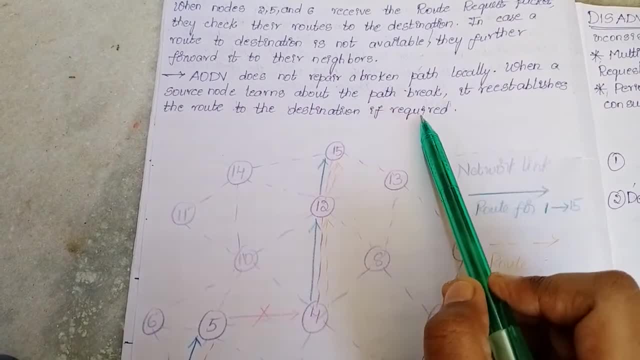 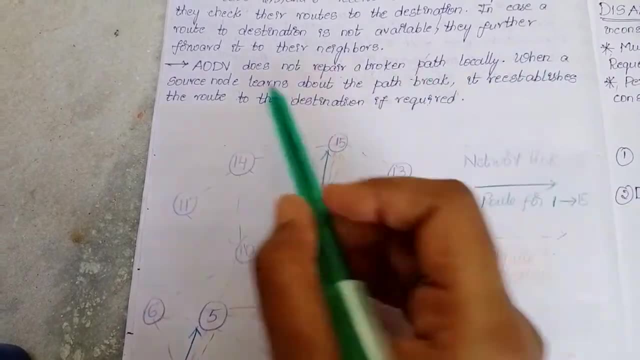 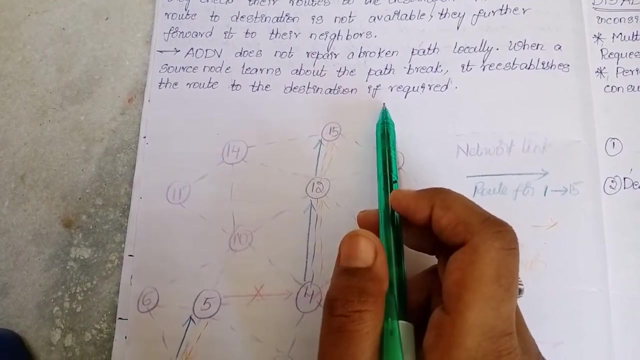 it re-establishes the route to the destination if required. aodv- actually dsr- also cannot repair its broken path locally. when a source node learns about the path break, it re-establishes the route to the destination if required, because a path break will always modify the route right from. 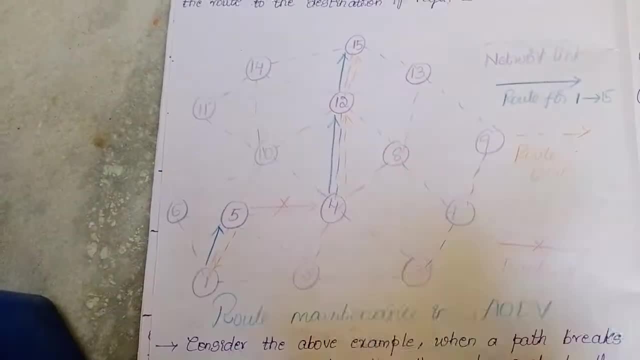 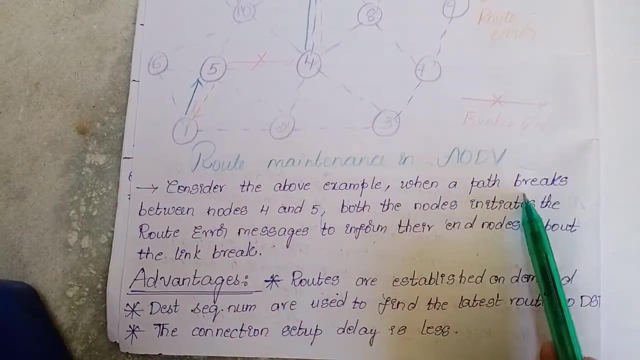 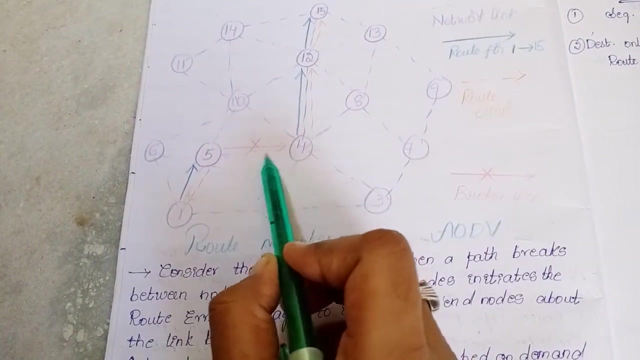 the source to the destination. c. consider the above example. this example: root maintenance in aodv. when a path breaks between nodes 4 and 5, this is node 4. this is node 5. when the path break, path break, broken link is indicated by an into mark like this: 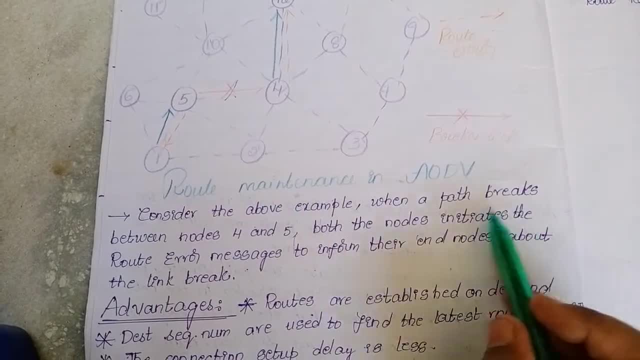 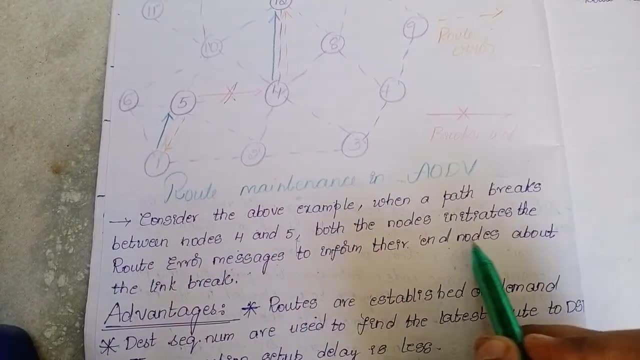 consider the above example. when a path breaks between nodes 4 and 5, both the nodes initiates the root error messages to inform their end nodes about the link break. that means if a path breaks between nodes 4 and 5, both the nodes initiate the root error messages to inform their end nodes. 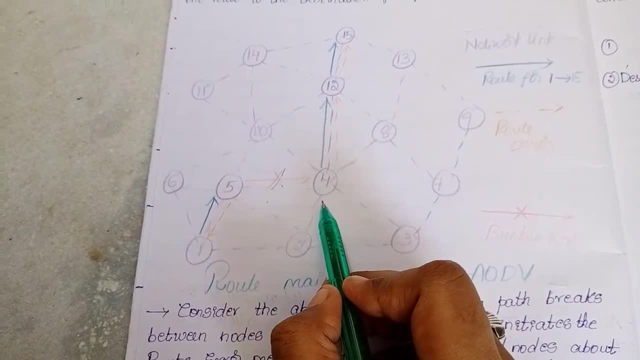 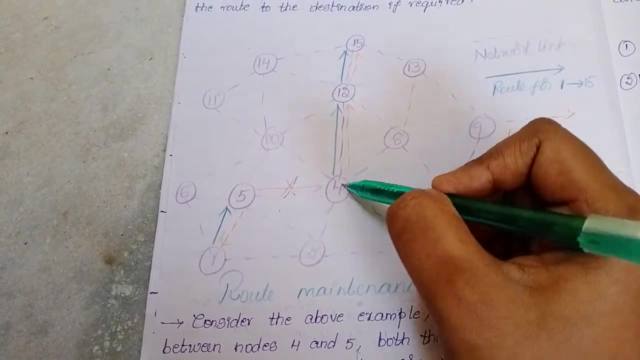 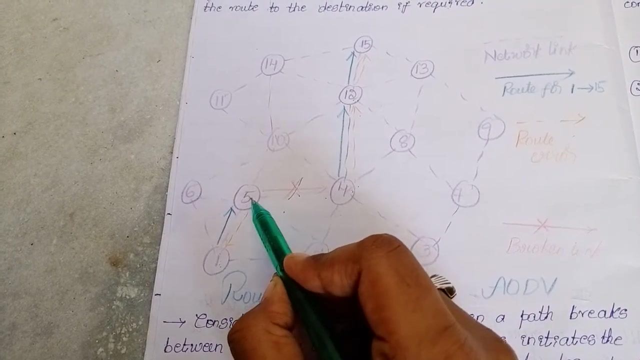 in these two nodes, then this will initiate a root error messages. here node 4 will initiate hit sniper means there is a root right, so it will indicate the end node. this is the end node for node 4. this is the end node for node 1. so this 5 will indicate will generate this root error. 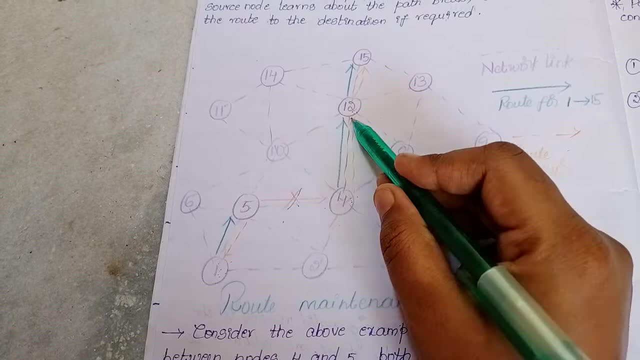 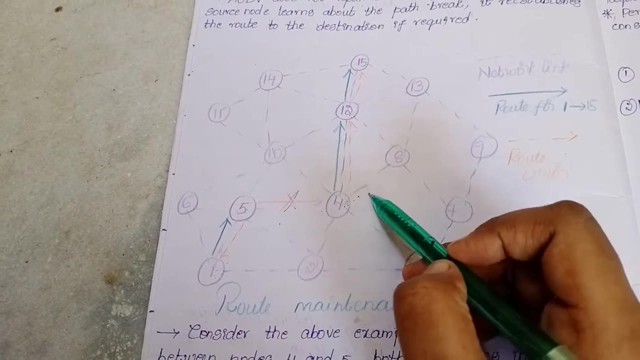 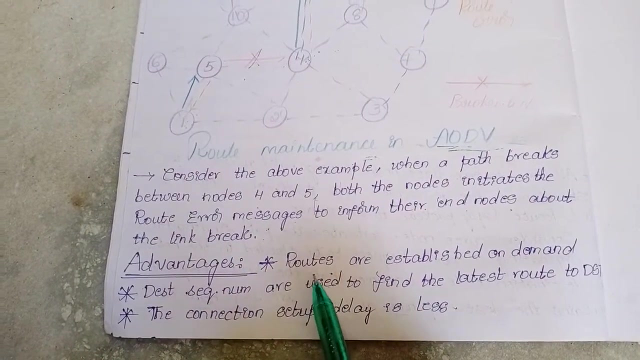 message to 1. this 4 will generate the root error message to 12. this is how root maintenance occurs in aodv. this normal dotted line indicates the network link between the nodes. so these are the advantages of aodv. routes are established on demand. destination sequence number. 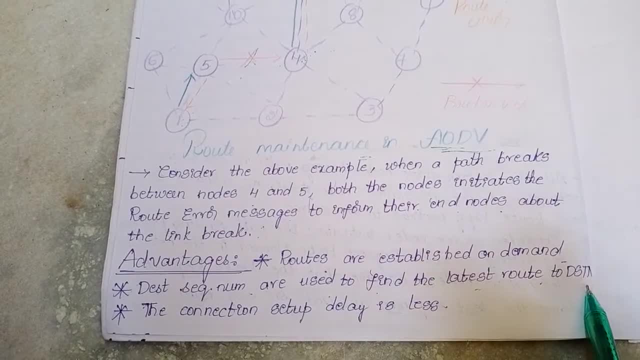 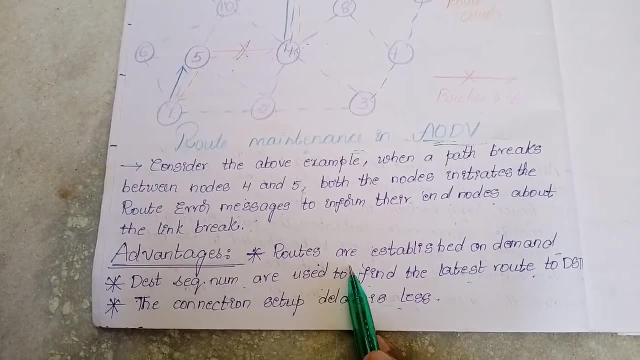 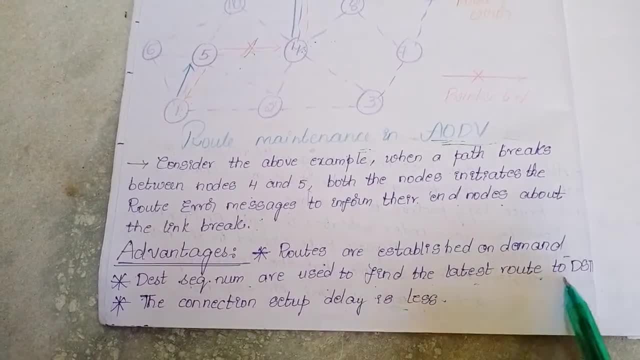 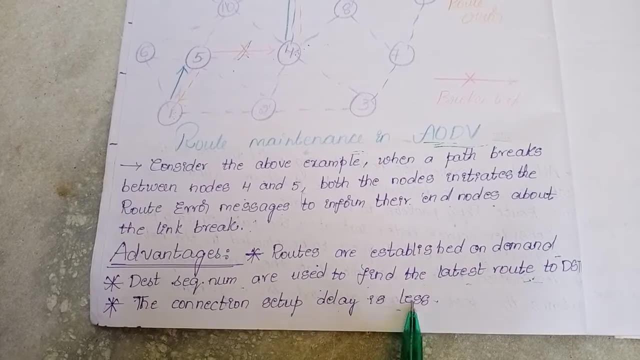 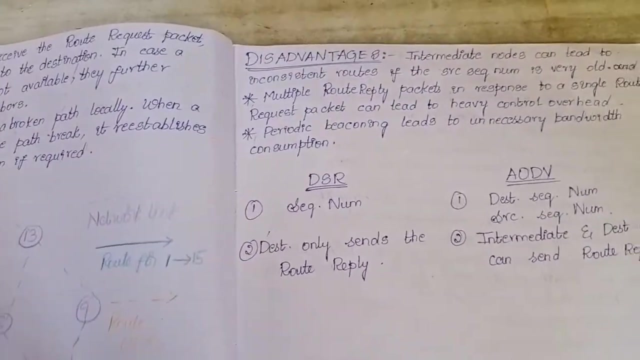 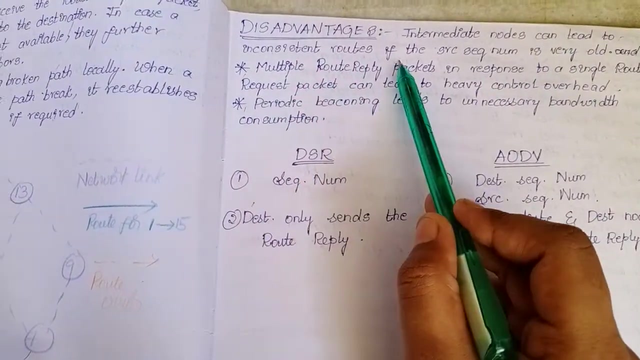 driven routing protocol. destination sequence number are used to find the latest route. in order to find the latest route, they use the highest sequence number value. the connection setup. delay is less. these are the disadvantages. intermediate nodes can lead to inconsistent routes if the source sequence number is very old. intermediate nodes means the 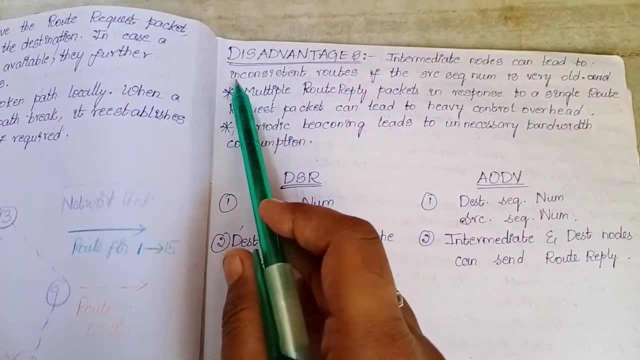 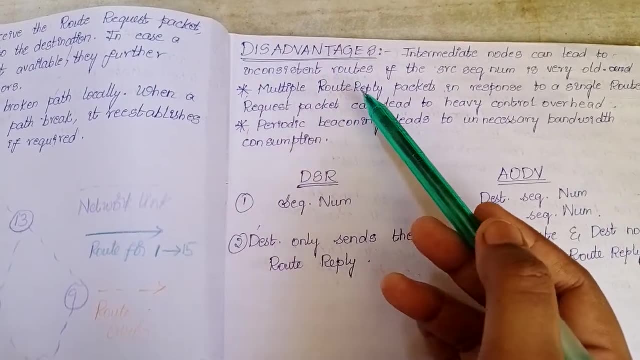 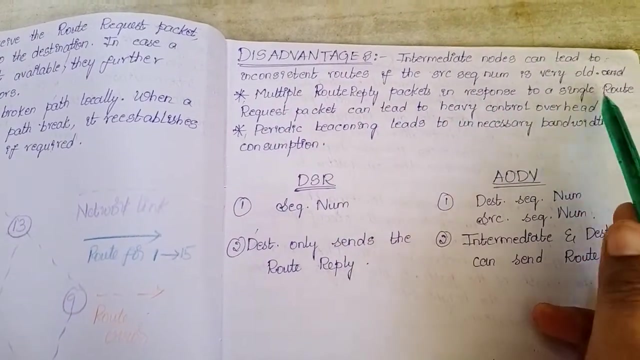 nodes between the service and the destination. it will read to the. it will lead to the. inconsistent routes means a not a good one. they might have broken links, like that if the source sequence number is very old. multiple route reply packets in response to a single route request packet can lead to heavy control. 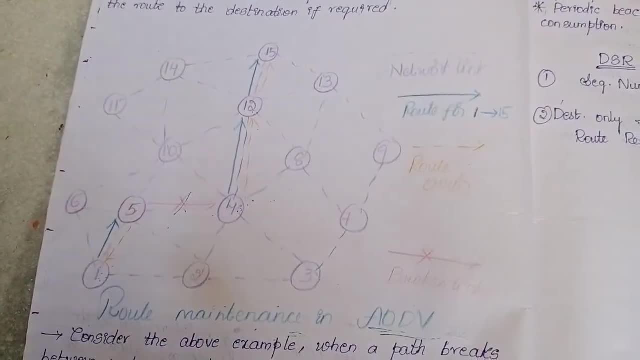 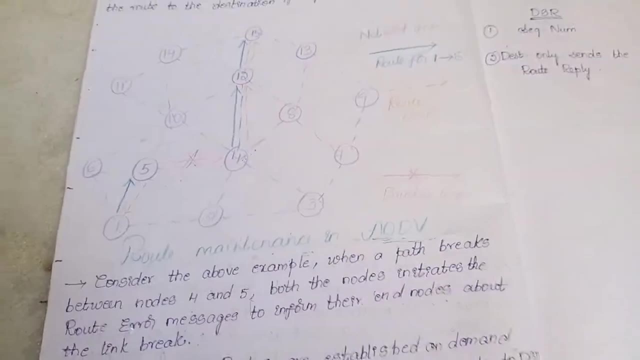 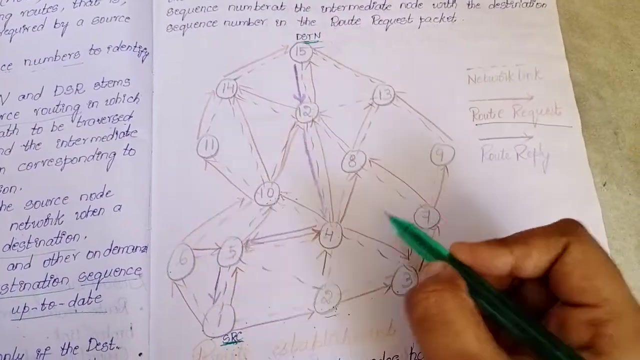 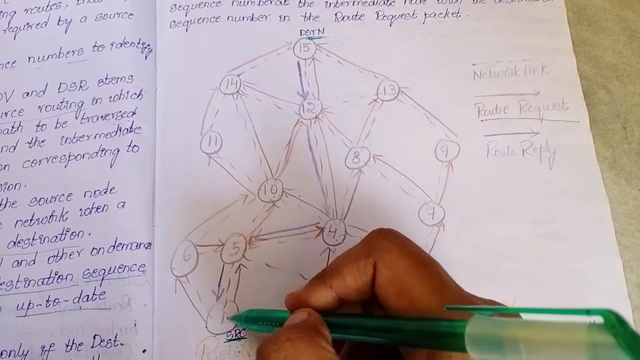 overhead. this means I'll tell with an example. for example, let us consider there is no broken link here, or we'll take the first one here. for example, if both 10, node 10 and node 4 have valid route to the destination, then they both will send the route reply packet to the node 1, right? 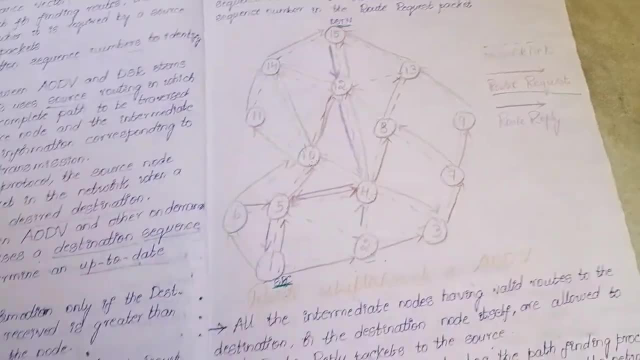 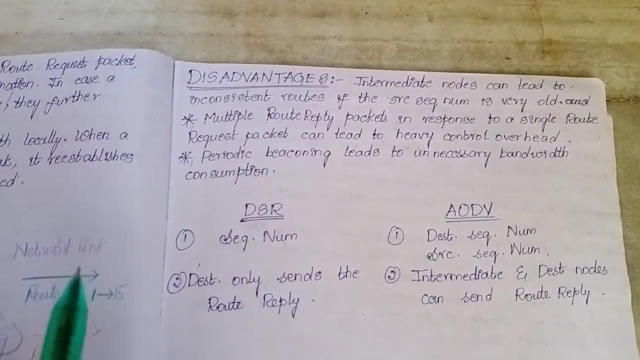 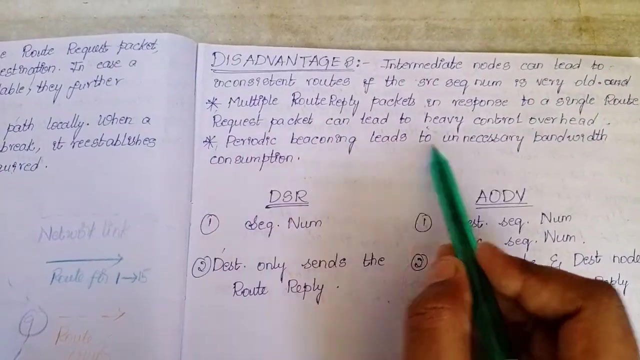 so it will create a overhead problem. right both intermediate nodes has sent the route reply packet to the source node. at a time it will come. it will be a heavy problem because it is running a heavy control overhead. it will lead to that right. periodic weakening leads to unnecessary bandwidth consumption. beaconing means hello packet, hello, we'll say.